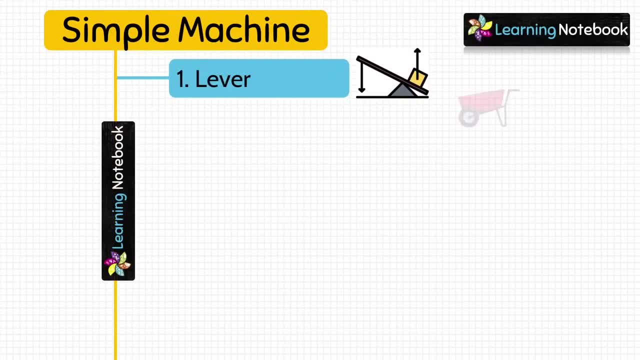 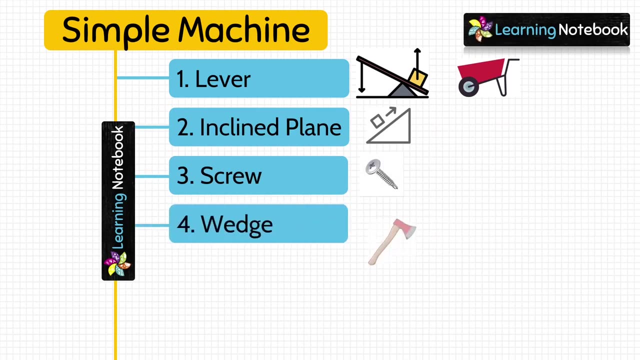 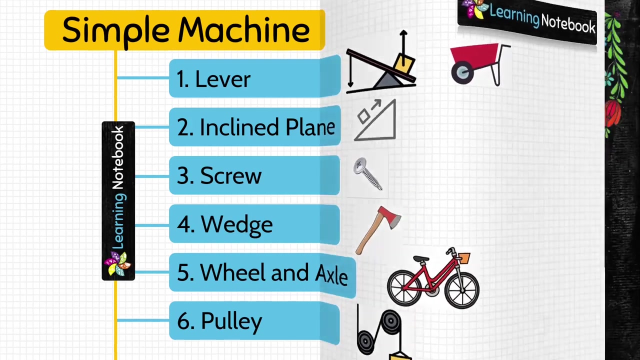 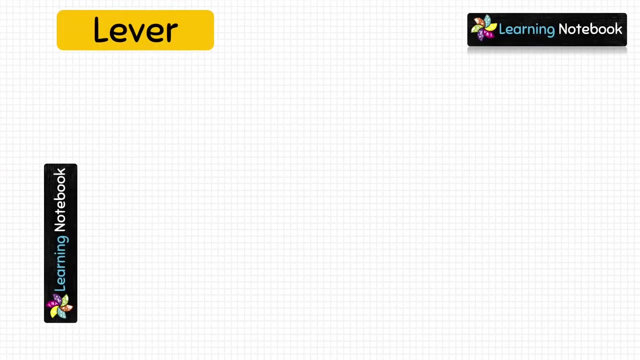 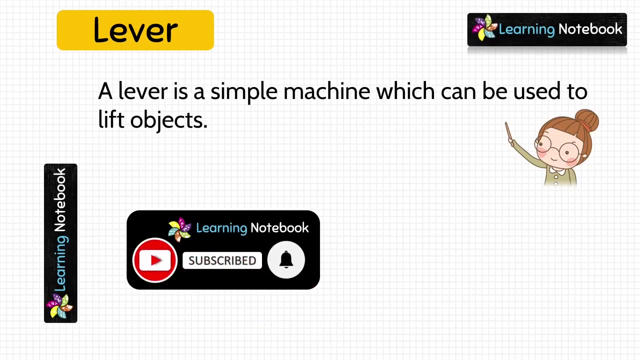 Students. there are six types of simple machine. They are lever, incline plane, screw, wedge, wheel and axle and, lastly, pulley. Let's learn each of them one by one. First, let's understand Lever. A lever is a simple machine which can be used to lift objects. 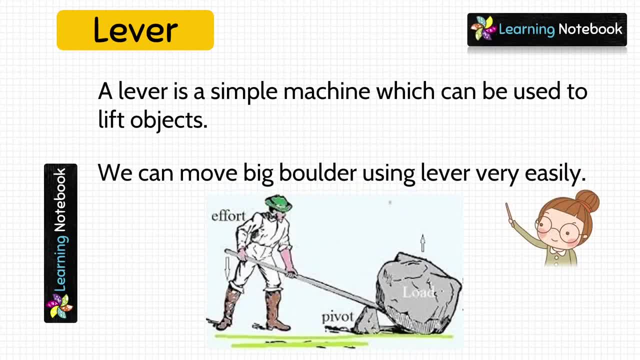 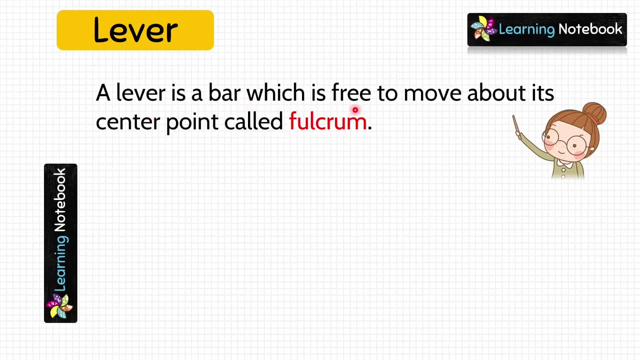 For example, we cannot move big boulder with our hands, But we can move it using lever very easily. So lever is a bar which is free to move objects. It is free to move about its center point, called fulcrum. Let's understand this with the help of a diagram. 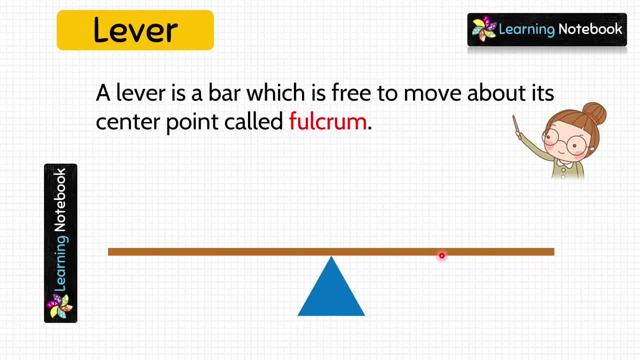 See, this is a bar. Let's read the definition once again. A lever is a bar, So this is a bar here in this diagram And definition says it is free to move about its center point, called fulcrum. So here this center point is fulcrum. 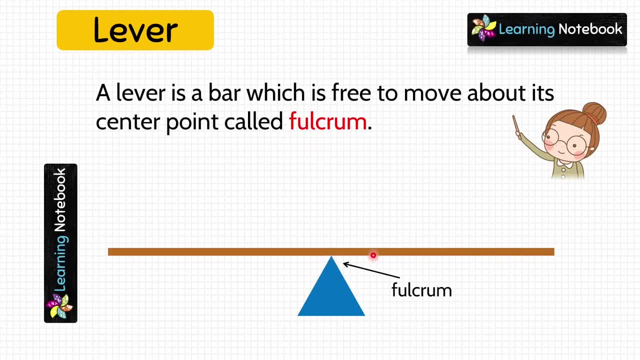 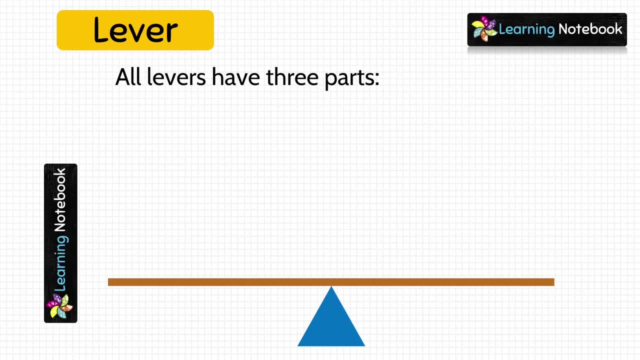 And this bar can move about fulcrum easily. All levers have three parts. First is fulcrum. Fulcrum is the point on which lever is supported, Like here. this point Is fulcrum On which this bar lever is being supported. 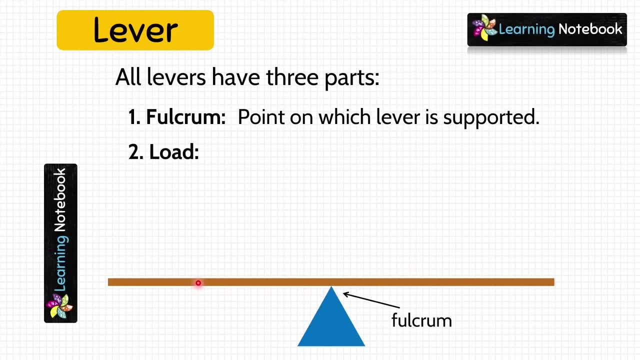 Next part of lever is load. It is the weight on which force is applied, Like here. this is the load. This is the weight on which force is being applied. Students, in our last example, last example, big boulder was the load. 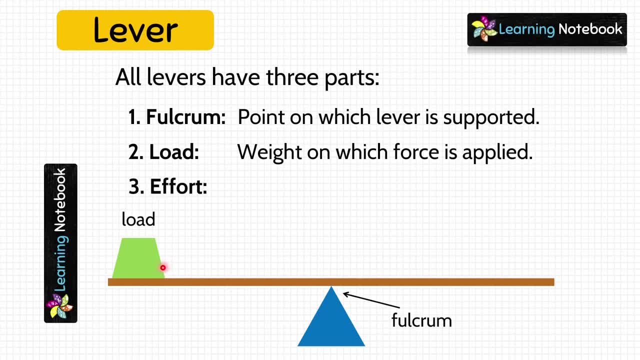 Right Now the third part. It is effort. What is effort? It is the force applied on lever. So here this is the effort, On the other hand of this bar, if we apply force on it, it is called as effort. 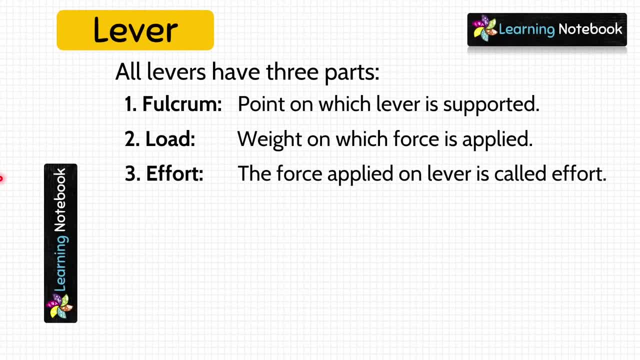 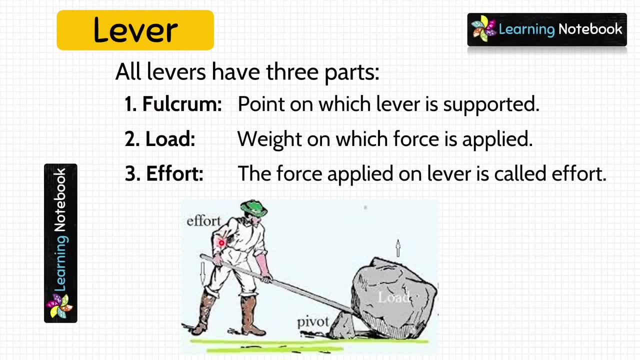 Let's understand these three parts again with the help of another example. Look at this picture. Here, this big boulder or stone is the load. Next, this point: It is fulcrum, Where the lever is being supported, And students. 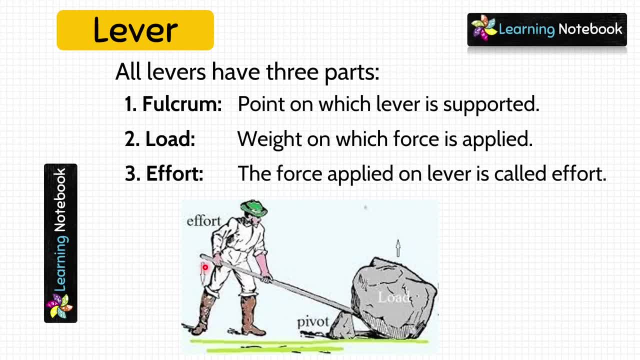 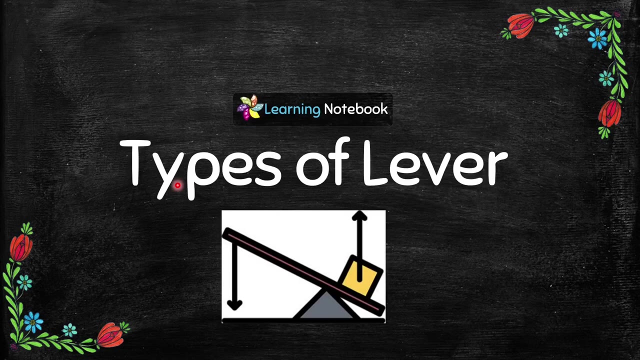 this man is applying force on the lever to lift the boulder. It is called as effort. So all levers have three parts: Fulcrum, load and effort. Now let's learn about types of lever. Levers are classified on the basis of: 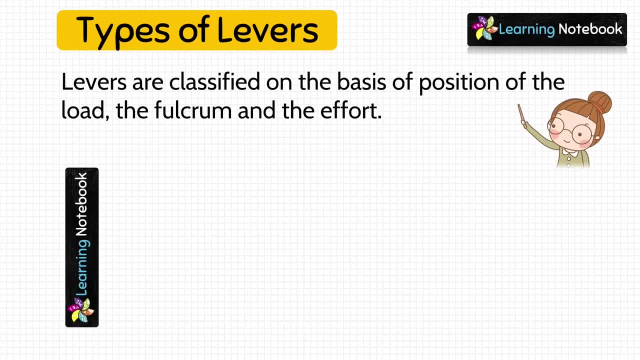 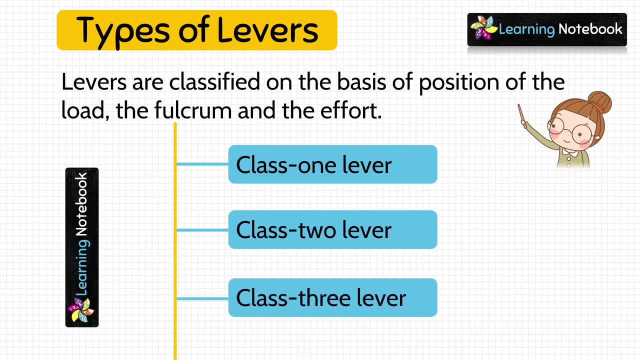 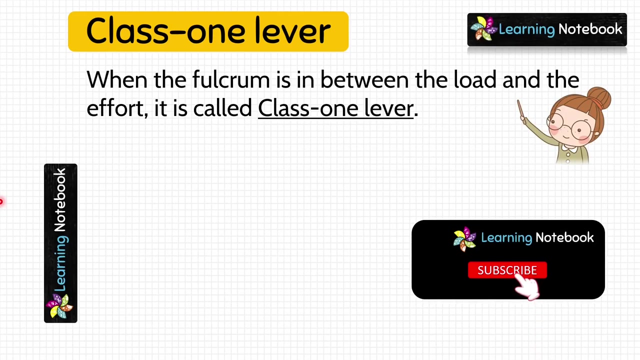 position of the load, the fulcrum and the effort. So there are three types of lever: Class I lever, Class II lever and Class III lever. Let's understand them one by one. When the fulcrum is in between the load and the effort: 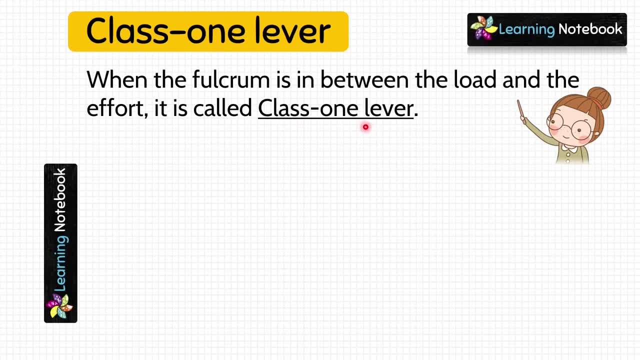 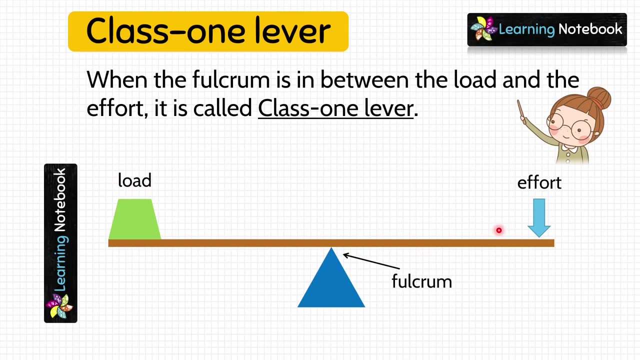 it is called as Class I lever. Let's understand this with the help of a diagram. See, this is a lever, And here this fulcrum is in between load and the effort. So this is Class I lever. Let's see some examples. 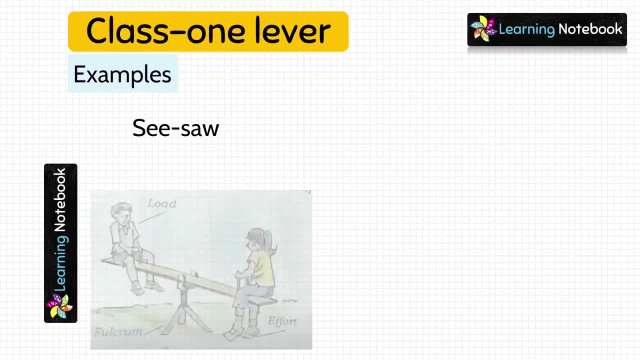 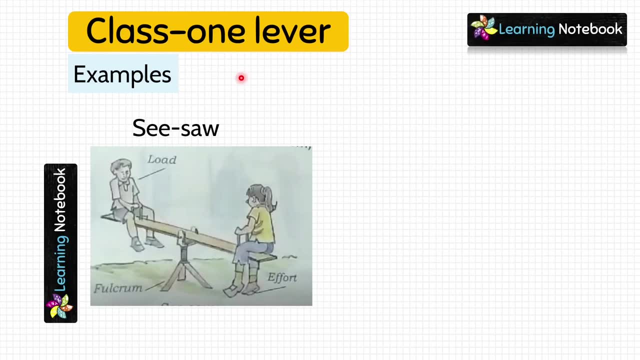 First example is seesaw. Seesaw is a very good example of Class I lever Because, as you can see, the fulcrum is in between load and the effort. One child is making the effort to lift another child. So this is an example of Class I lever. 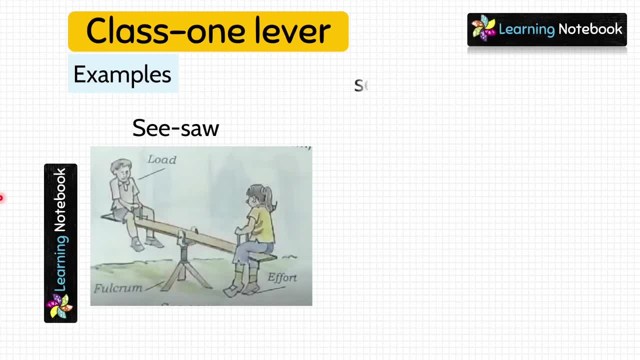 Another example of Class I lever is scissors. Here students in scissors, this is fulcrum. Then on this end we put load and on another end we make effort. So scissors are also example of Class I lever. Another good example of Class I lever is nail cutter. 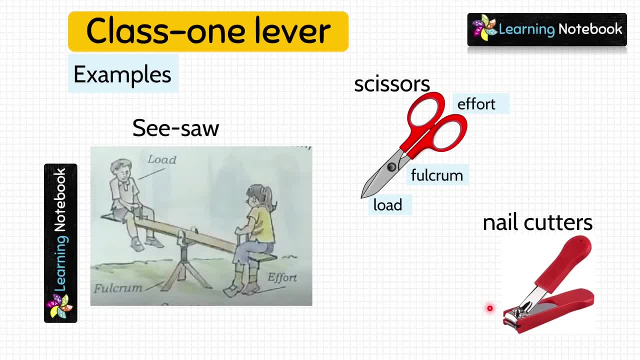 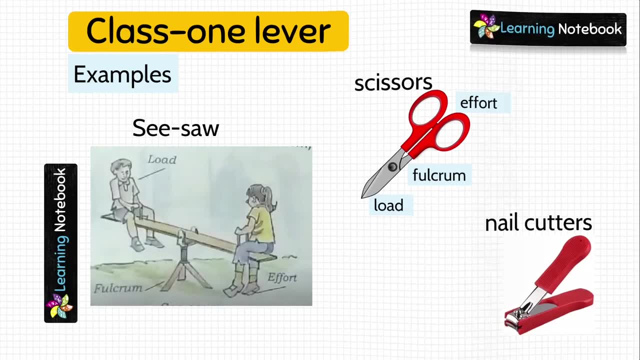 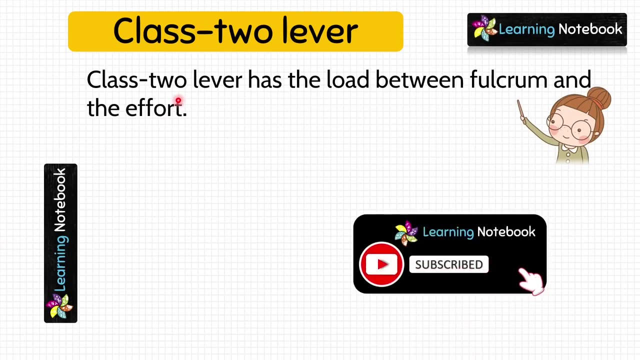 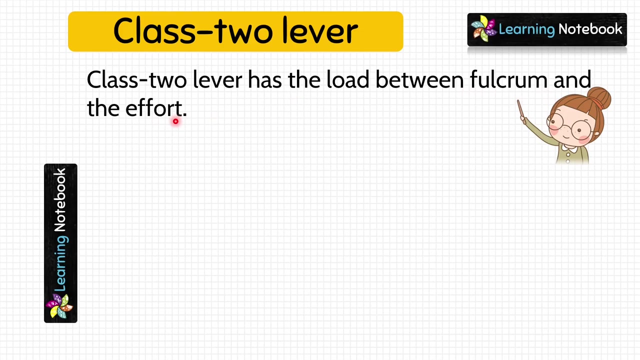 Okay, students now. do you know any other example of Class I lever? Do tell me in the comment section. Now let's learn about Class II lever. Class II lever has the load between fulcrum and the effort. Let's understand this with the help of a diagram. 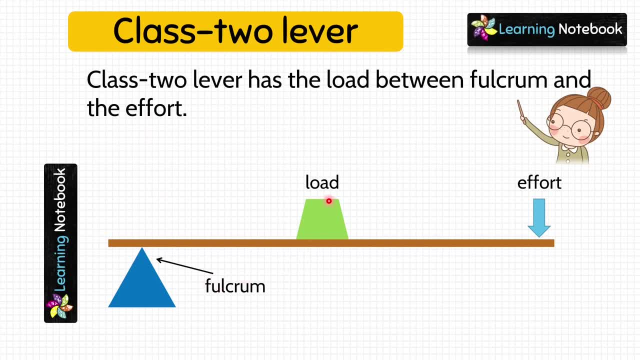 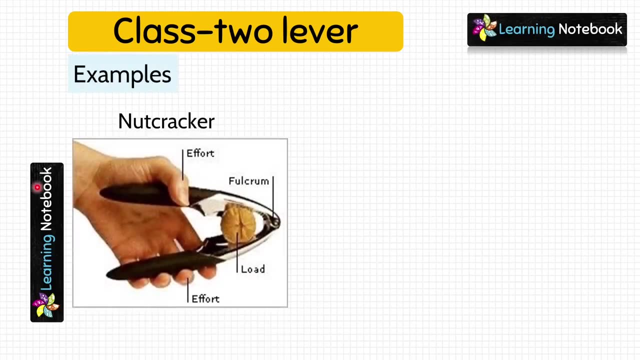 Here the load it is in between fulcrum and the effort. Let's see examples of Class II lever. First example of Class II lever is nutcracker. Look here, students, this is the fulcrum. Here we are putting nut. 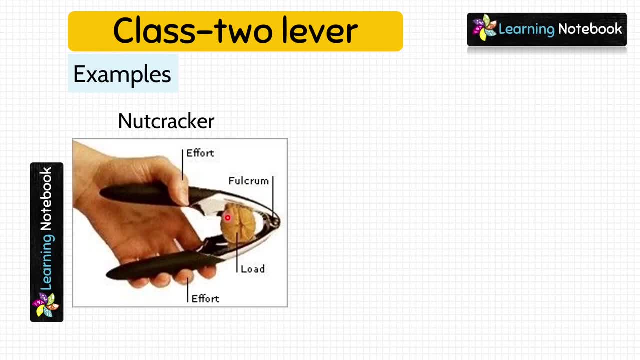 that is load in the middle. and here we are making the effort to crack this nut. So load is in between fulcrum and the effort, Right? Let's see other example of Class II lever Bottle opener. Here can you tell me where is the fulcrum? 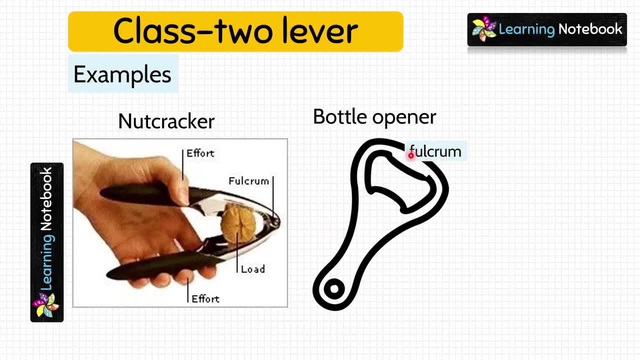 Yes, This is the fulcrum. Then here we put the load, which is the cap of the bottle, and then here we make the effort to open that bottle. And then- other example of Class II lever is wheelbarrow, Here also. 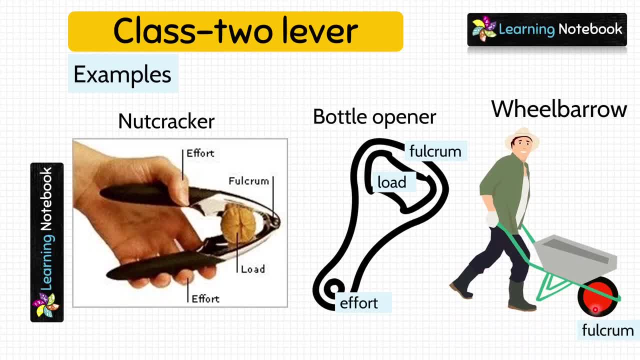 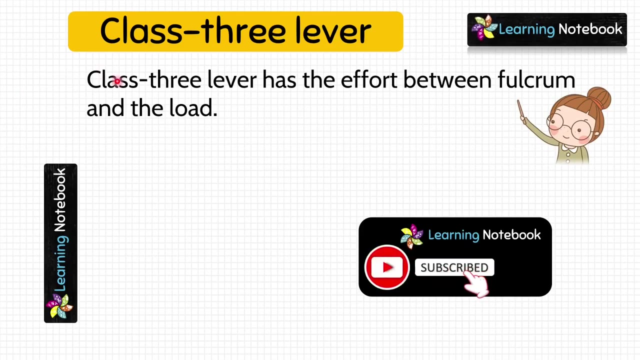 this is the fulcrum. Then in the middle we put the load, And then here we make the effort to carry that load. So all these are examples of Class II lever. Now what is Class III lever? Class III lever has the effort. 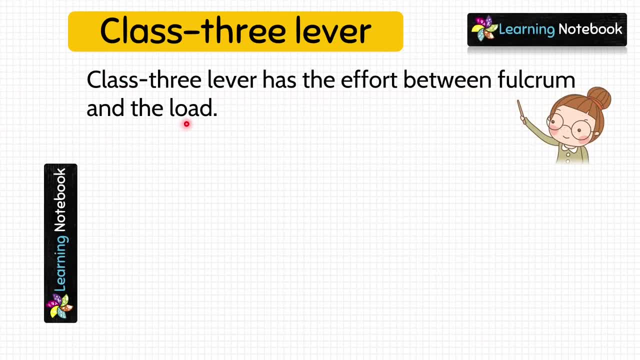 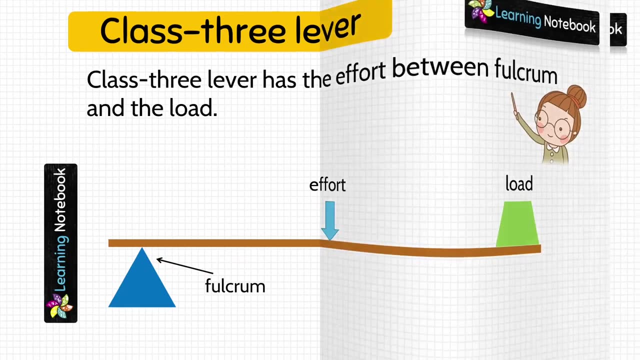 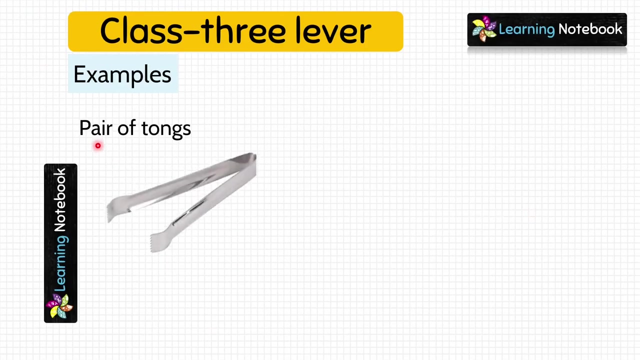 between the fulcrum and the load. Look at this diagram. Here the effort is in between fulcrum and the load. So this is Class III lever. Let's see some of its examples. First example is pair of tongs. 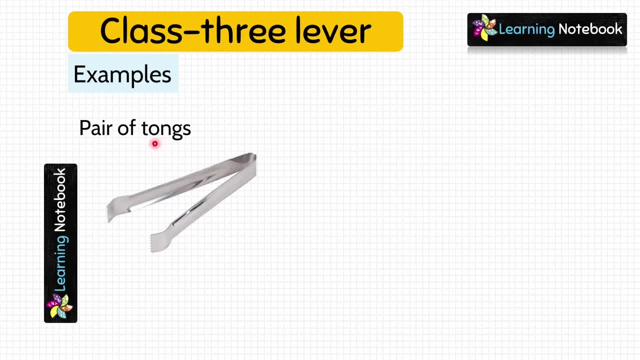 Students, you must have seen this in your kitchen. In Hindi we call it chimta. So here in tongs we have fulcrum. Then on this other end we put load like chapati, And in the middle 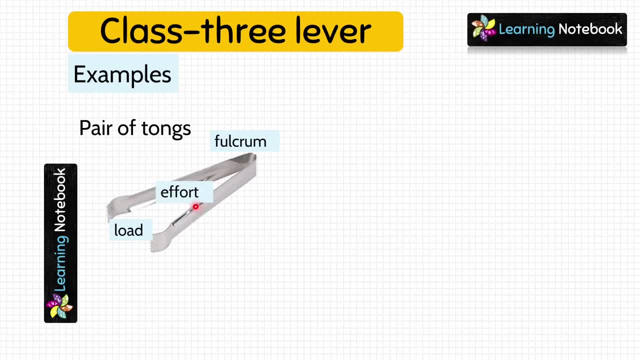 we make effort to hold that chapati. So pair of tongs is an example of Class III lever. Similarly, students forceps or tweezers- they are also examples of Class III lever, Because here also effort is in between. 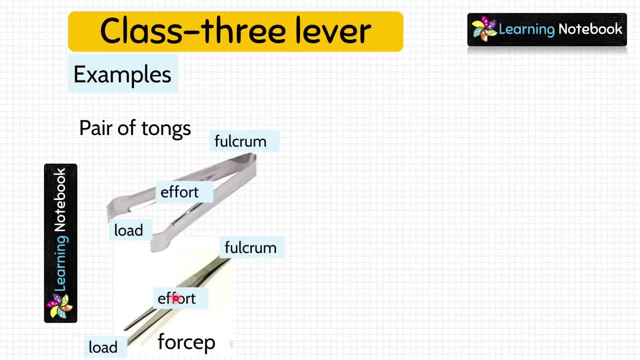 fulcrum and the load. Let's see more examples of Class III lever Broom. Look here, students. This is the fulcrum in broom. Then on this other end we have load like garbage And in the middle 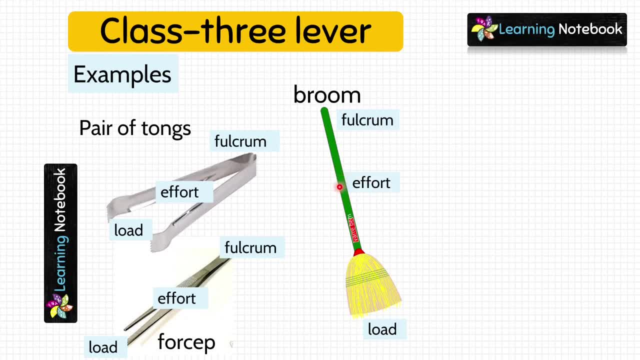 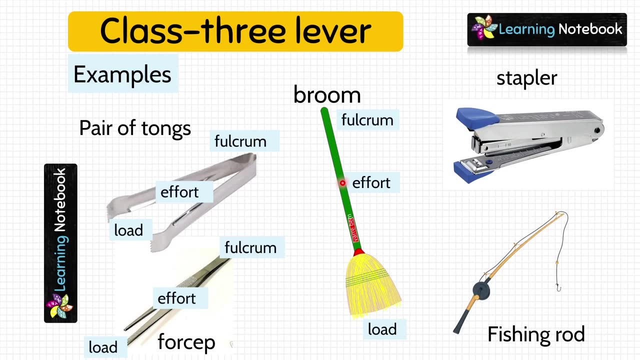 we make the effort. So broom is also an example of Class III lever. Other examples are stapler fishing rod. All these are examples of Class III lever. Now, students, can you tell me more examples of Class III lever in the comment section? 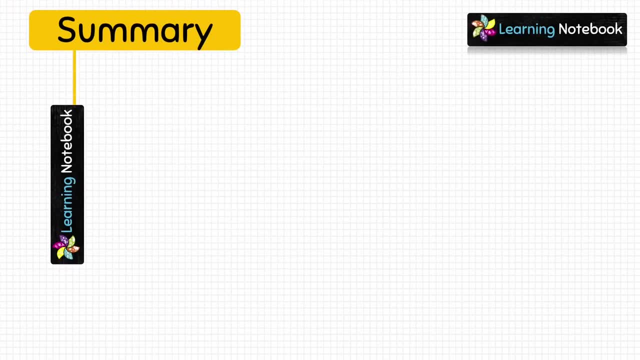 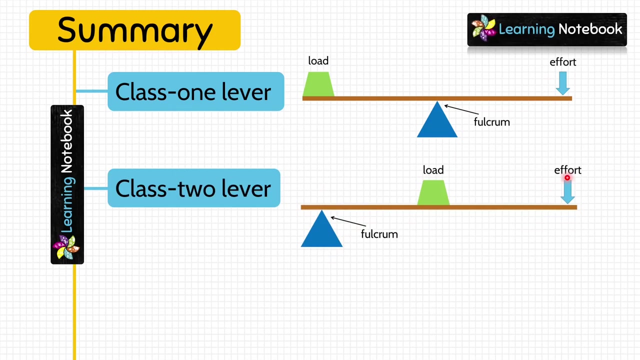 So, students, we learnt three types of levers. Let's revise them. Class I lever: Here fulcrum is in between load and the effort. In Class II lever, load is in between fulcrum and the effort. And in Class III, lever. 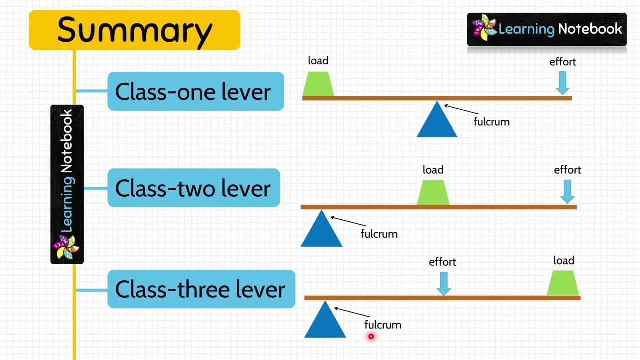 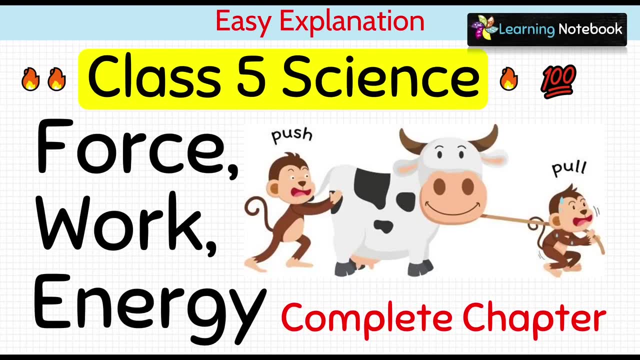 effort is in between fulcrum and the load. Students, we would like to tell you that we also have a separate video on complete chapter of work force and energy for Class V. I would recommend you to watch this video as well. You will find its link. 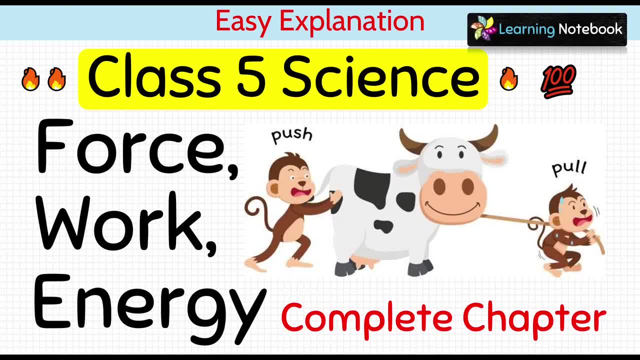 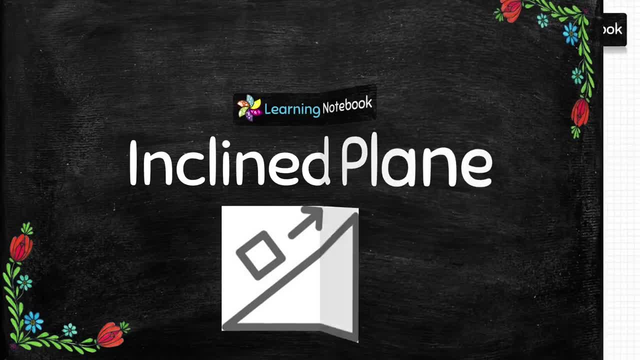 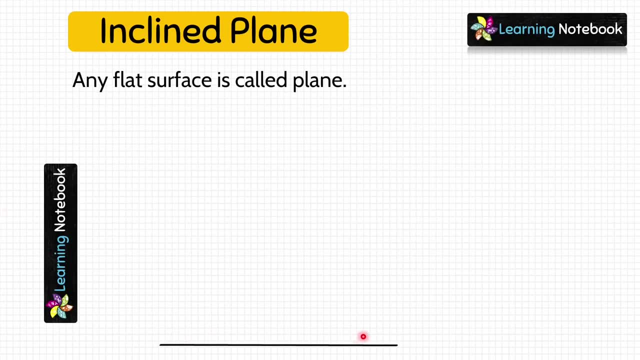 here on the top and below in the description box. Now let's move to our next topic: inclined plane Students. any flat surface is called a plane. Like this: this flat surface is a plane. Now, when this plane surface is slanted, 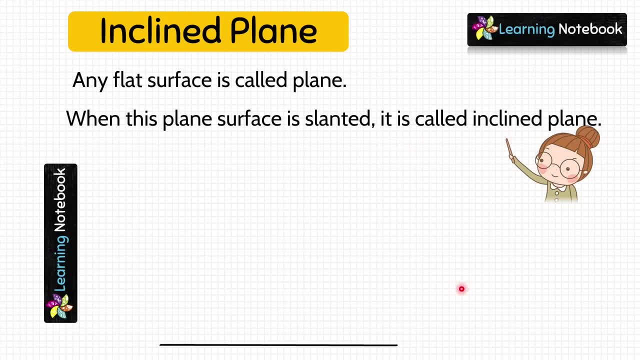 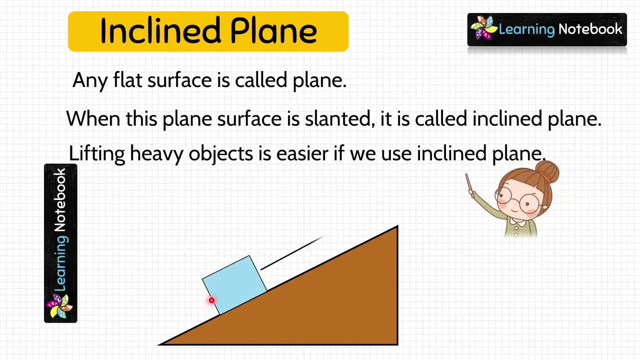 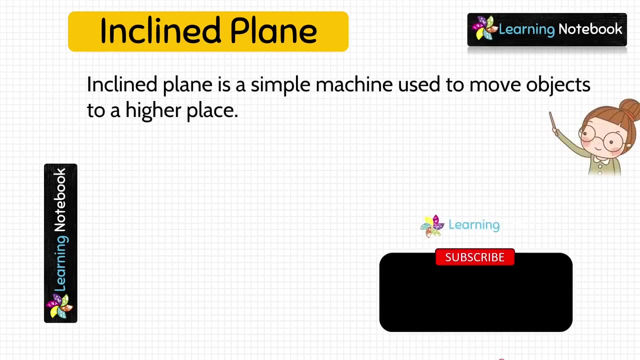 it is called as inclined plane, Like here, if we slant this plane surface, it has become an inclined plane now, And lifting heavy objects is easier if we use inclined plane. So let's learn more about inclined plane. So what is inclined plane? 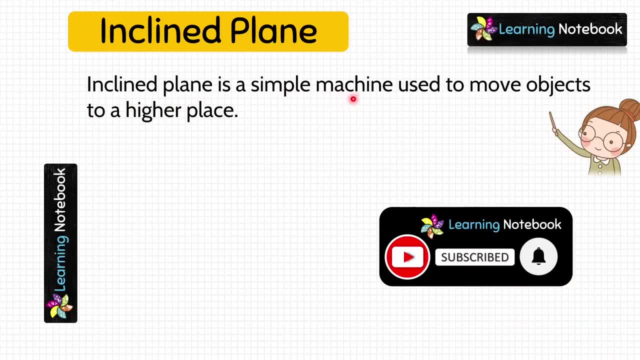 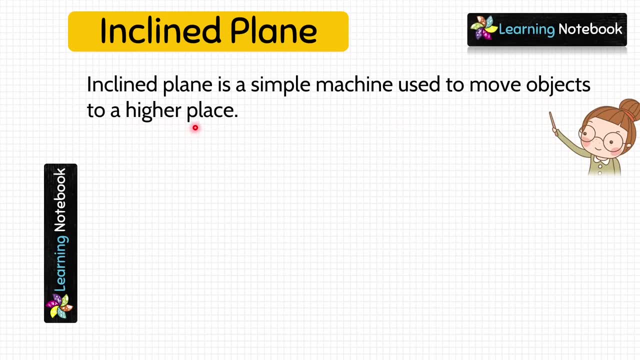 Inclined plane is a simple machine used to move objects to a higher place. Let's understand this with the help of a diagram, Students. this is an inclined plane. Now, if we want to move this object, this blue object, from this point. 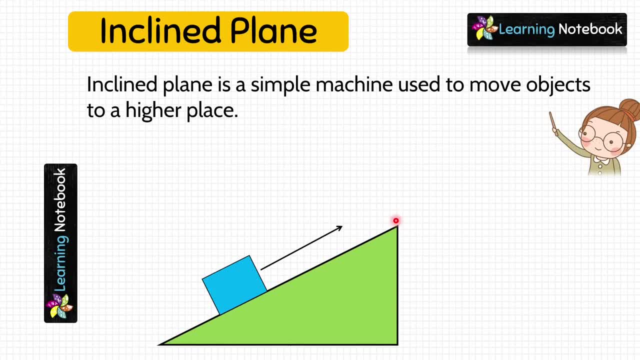 to this point it will require large amount of effort. But if we use inclined plane to move this object towards top, it will require very less effort. So inclined plane is a simple machine used to move objects to a higher place. Some examples: 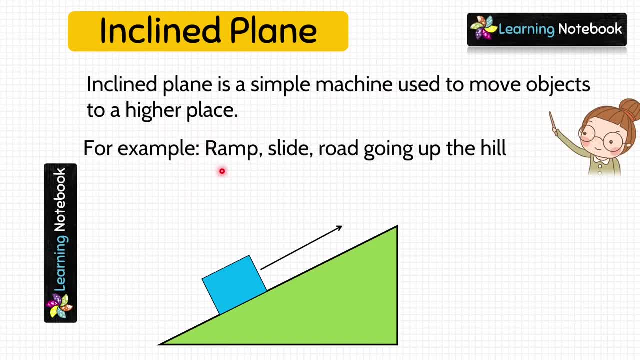 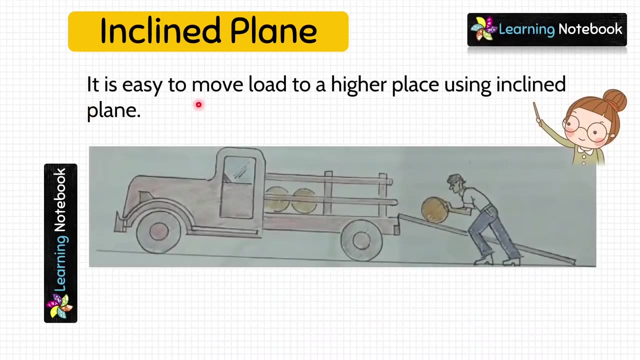 of inclined plane are ramps. Ramps are usually made in hospitals to use wheelchairs, Then slides, road going up the hill. All these are examples of inclined plane. So, students, as I told you, it is easy to move load. 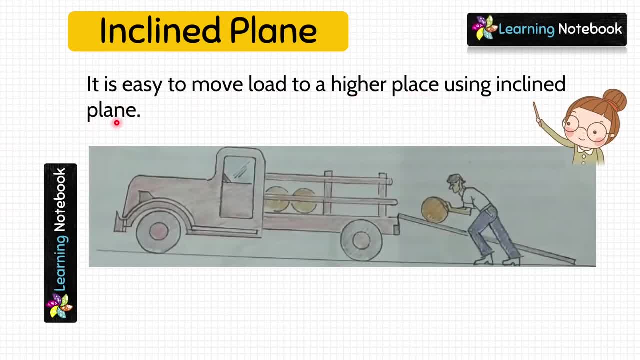 to a higher place using inclined plane. Look at this picture. This person has to move all these drums in the truck. If he lifts them and put them in the truck, it will require large amount of effort, But if he rolls them up using inclined 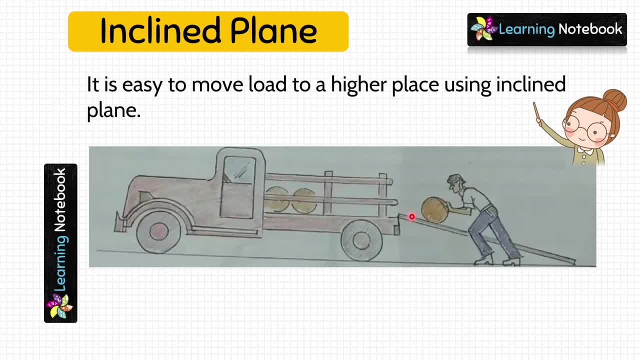 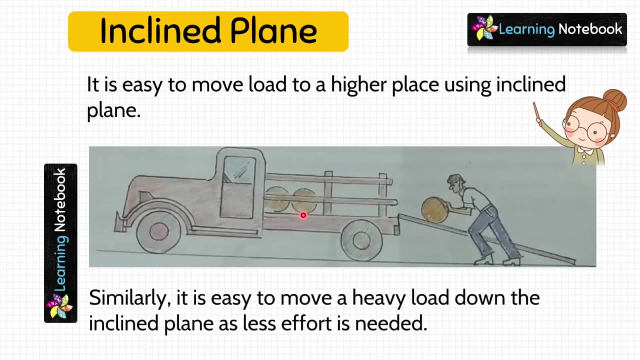 plane as shown in this picture, it will require very less effort. Similarly, when this person has to unload all these drums, then also it is easy to move them using inclined plane. So it is easy to move a heavy load up and down. 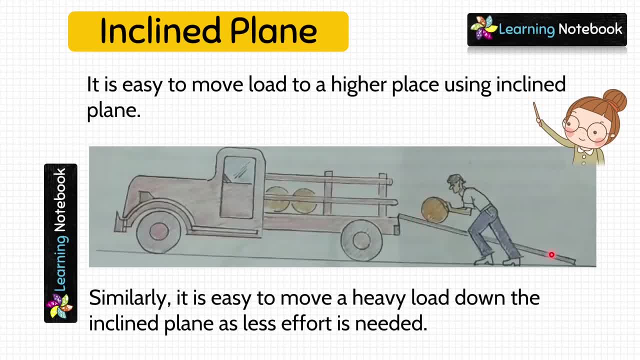 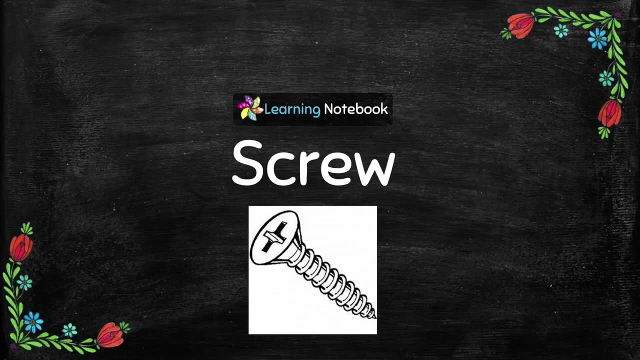 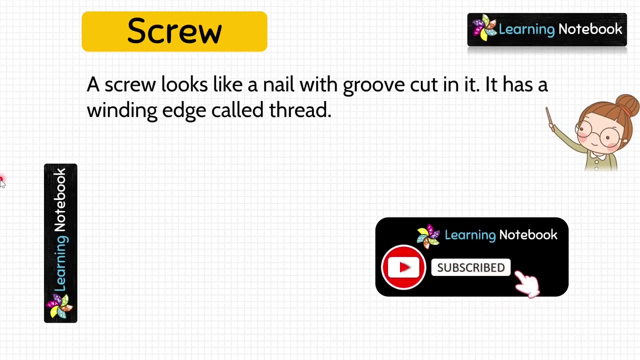 using inclined plane, as very less effort is needed. So, students, till now we have learnt two types of simple machines: lever and inclined plane. Now, next type of simple machine is screw. We use screws to join together many things around us. A screw: 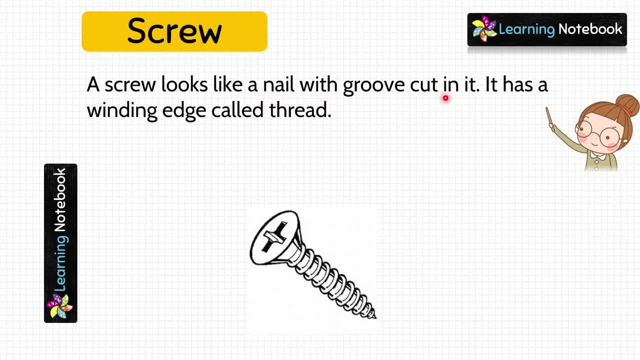 looks like a nail with groove cut in it. It has a winding edge called thread. So this is a screw, students, and this is called as winding edge, which is thread of the screw. Next, a screw is actually an inclined plane wrapped around a cylinder. 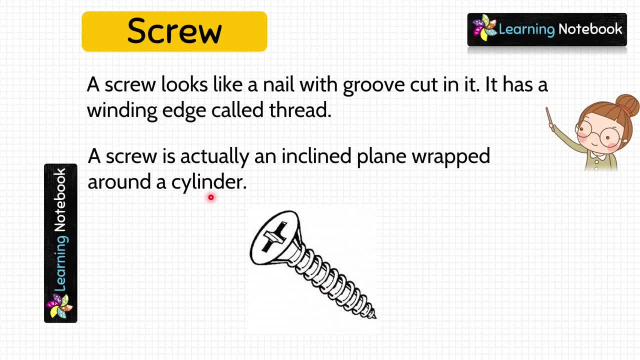 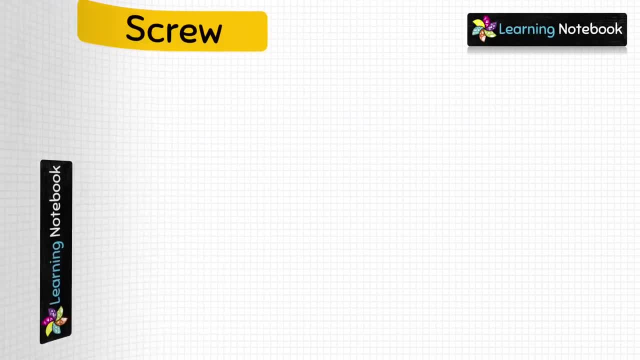 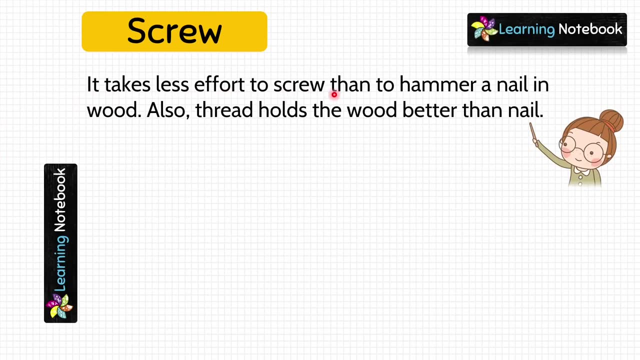 Students. I will explain this line in detail with the help of an activity in a short while. Also, it takes less effort to screw than to hammer a nail in the wood. Also, thread holds the wood better than a nail. So now we know why. 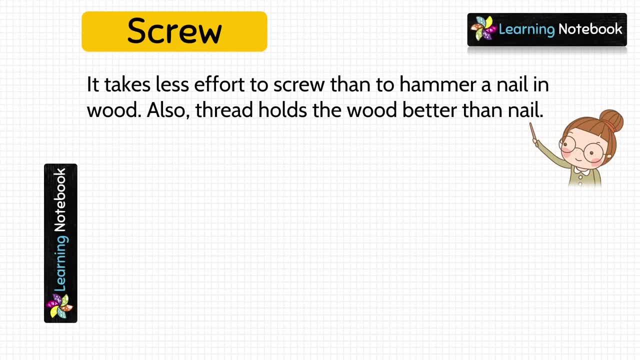 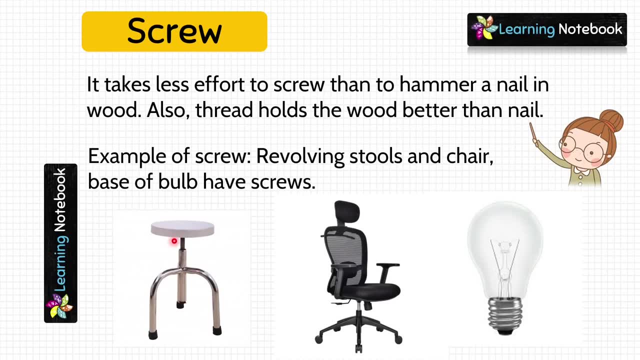 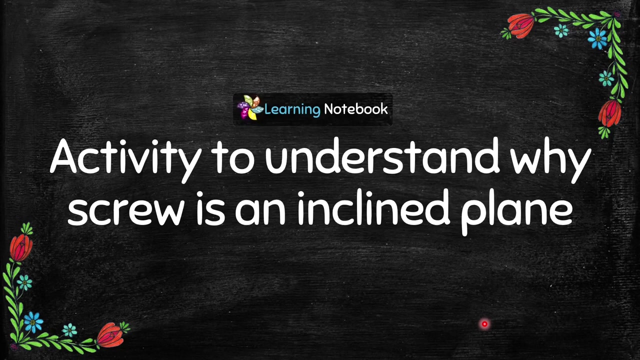 screw is better than a nail. Let's see some examples of screw: Revolving stools, revolving chair, base of bulb have screws. So all these are examples of screw. Now, students, let's do an activity to understand why screw is. 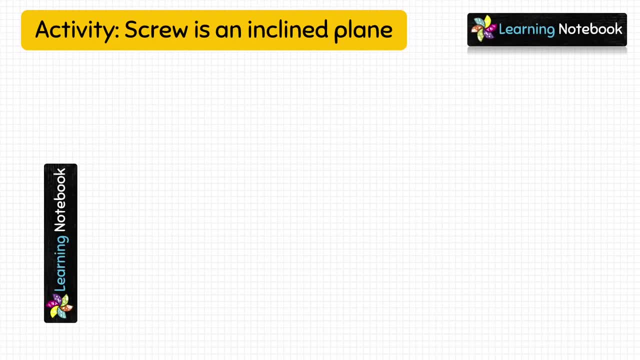 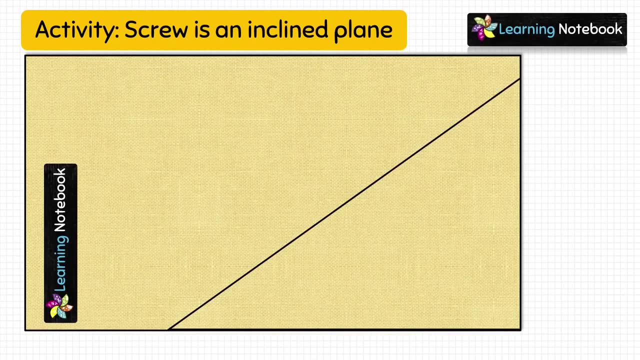 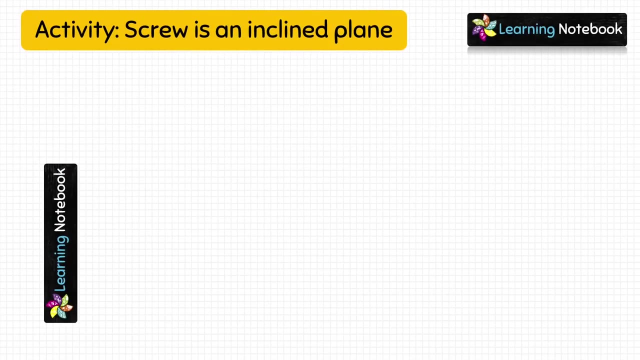 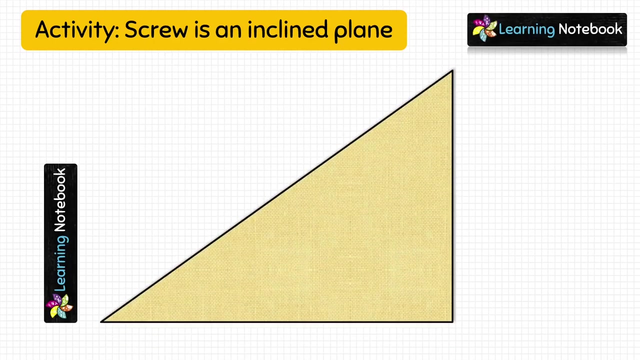 an inclined plane. Take one yellow sheet of paper and draw a triangle on it, Then cut it with the help of a pair of scissors. So this is the triangle, students, we have cut. Now let's colour its diagonal edge with a red coloured. 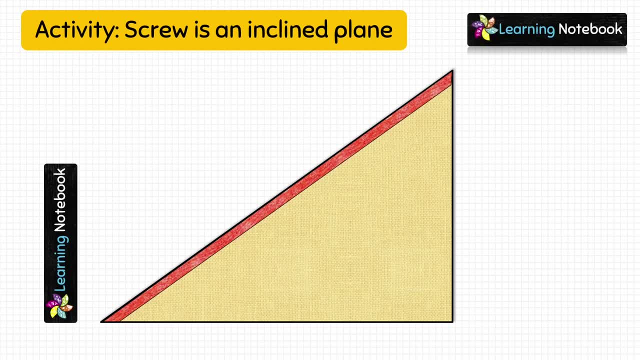 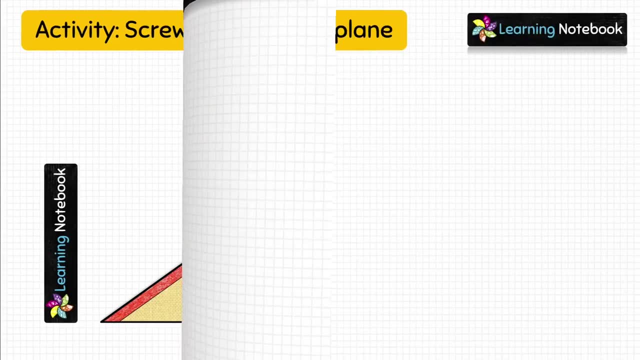 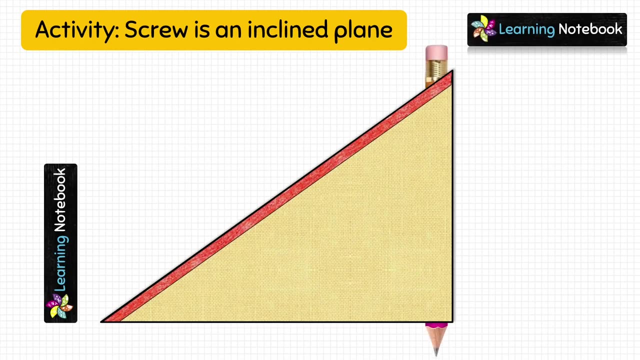 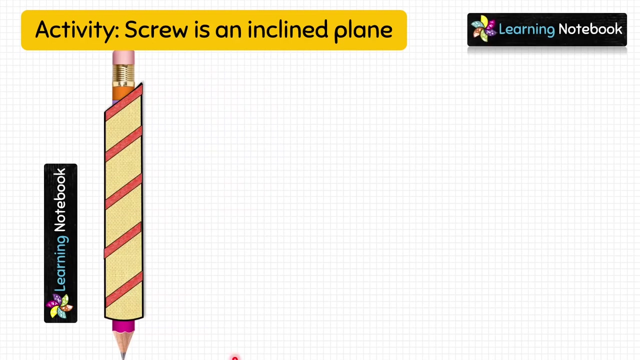 sketch pen, as shown here. So now, students, we have made an inclined plane. In the next step, take a pencil and start taping this inclined plane around the pencil as shown here. Students, make sure that the paper is tightly wrapped around. 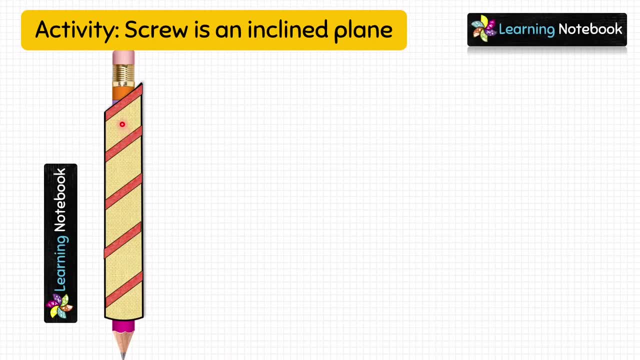 this pencil. Now observe that the diagonal red stripes are formed around the pencil. Here we have taken a pencil which is a cylinder and we have wrapped an inclined plane around it to form threads. These red stripes represent threads of the screw. Therefore we can say: 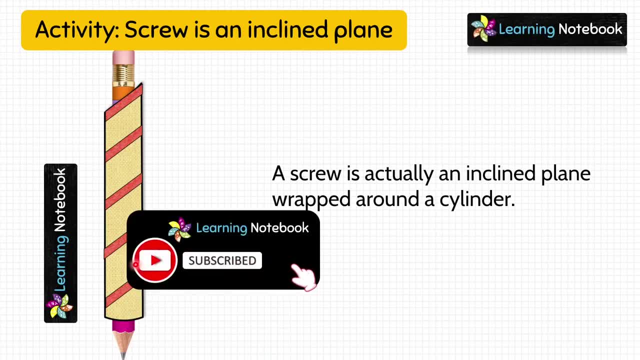 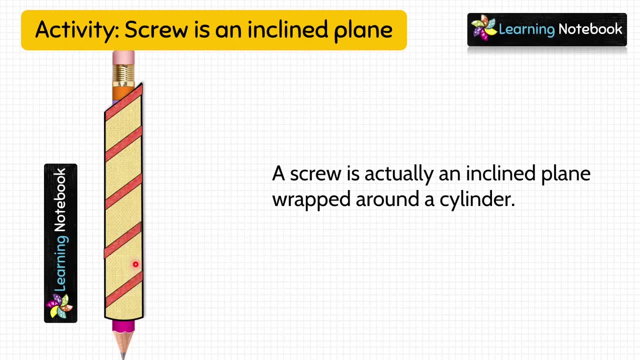 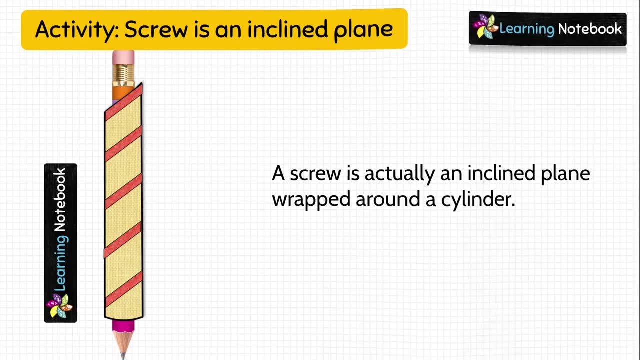 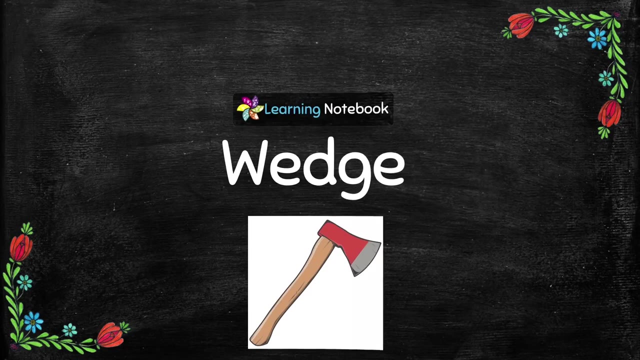 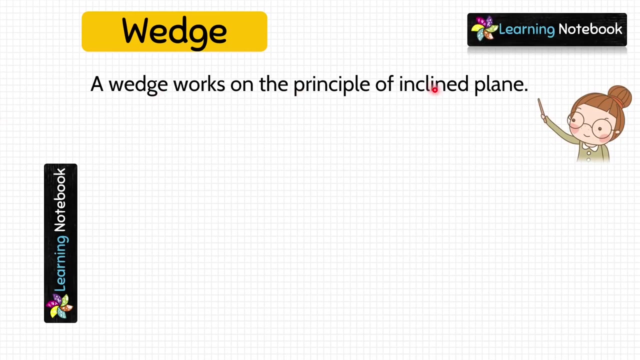 a screw is actually an inclined plane wrapped around a cylinder. So now, students, I am sure you have understood the meaning of this line: Screw is an inclined plane. Now, next simple machine is wedge. Our wedge works on the principle of inclined 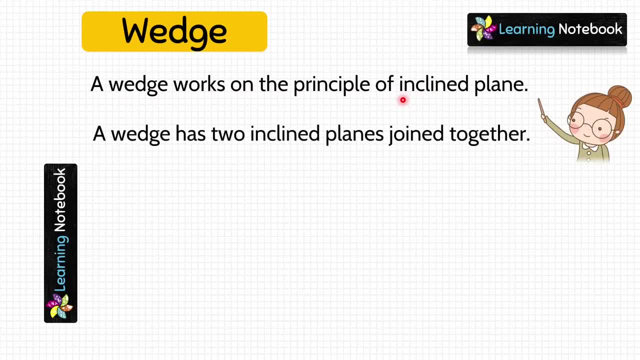 plane. A wedge has two inclined planes joined together. Let's understand it with the help of an example X. X is an example of wedge. X is used for cutting wood. Now let's see how this part of the X actually looks like. 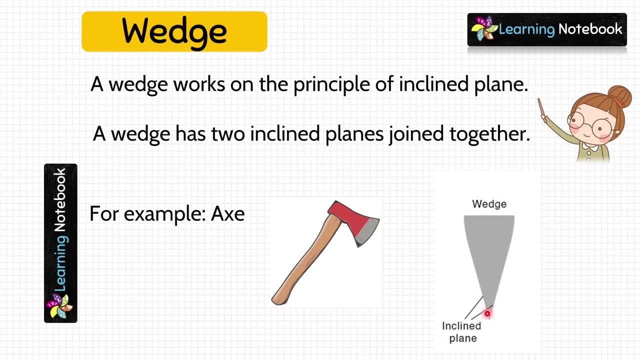 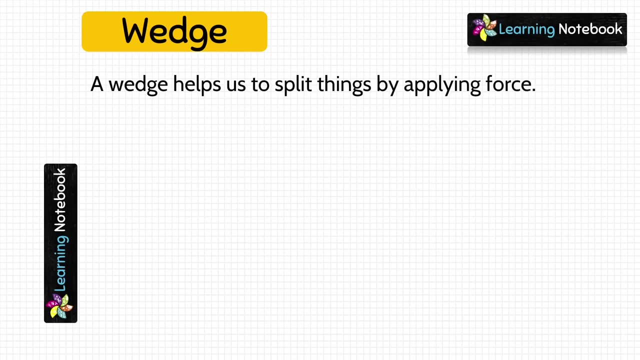 This is the part of the X and it has two inclined planes joined together And this is called as wedge. A wedge helps us to split things by applying force, Like X is used to cut wood, by applying force, Students sharp teeth are also. 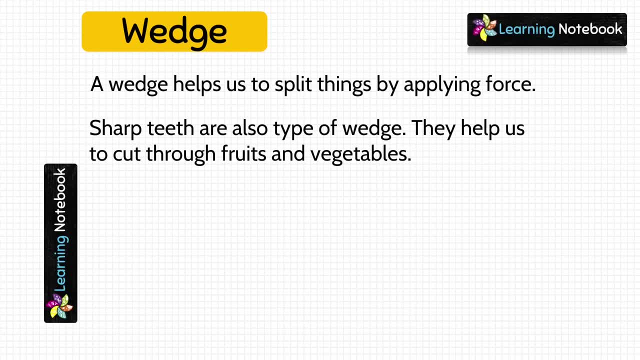 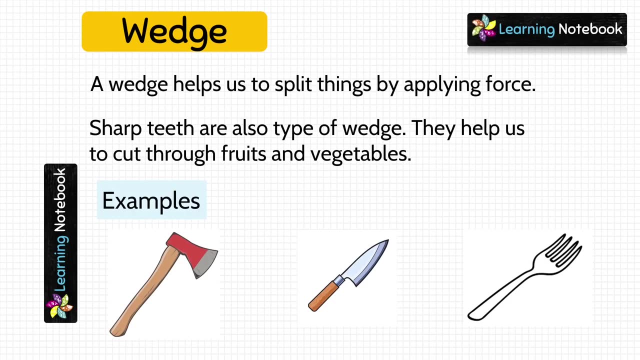 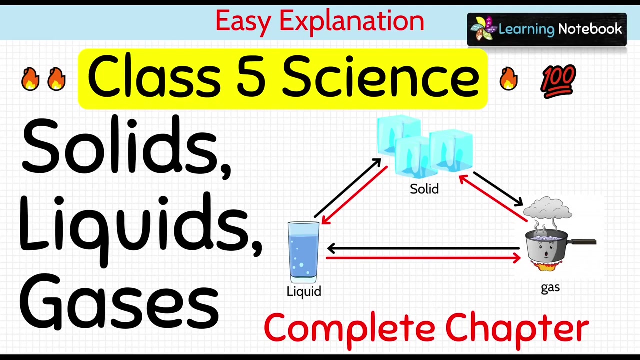 kind of wedge, because they help us to cut through fruits and vegetables, hence working like a wedge. Apart from X, other examples of wedge are knife fork, etc. Now, students, we also have a separate video on complete chapter of solids. 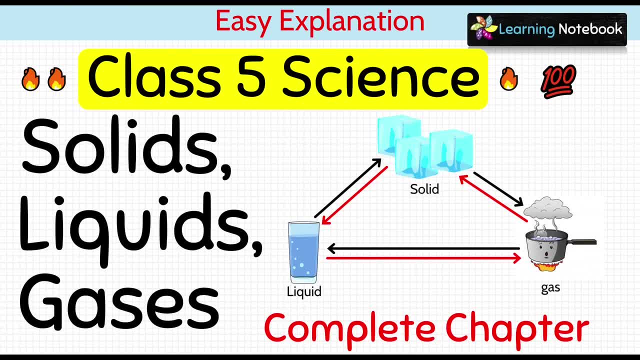 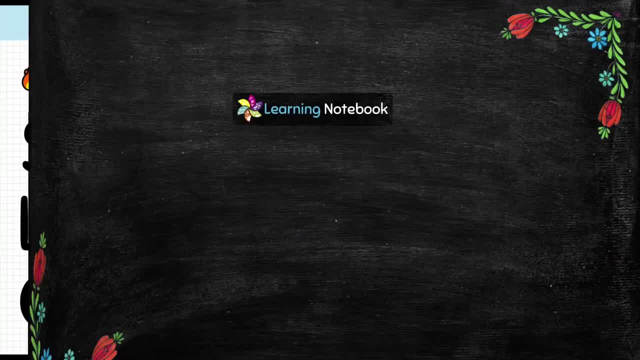 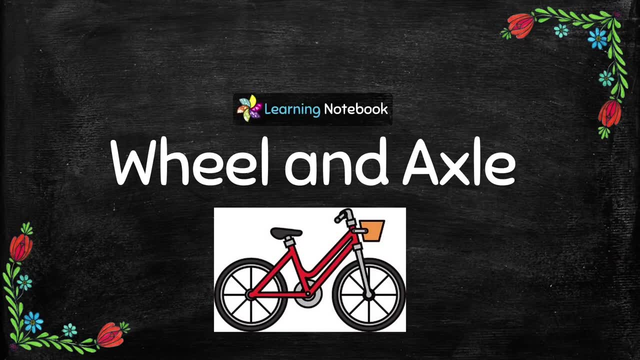 liquids and gases for class 5.. You will find the link to this video here on the top and below in the description box. So till now, students, we have learnt four kinds of simple machines: Lever, inclined plane, screw and wedge. 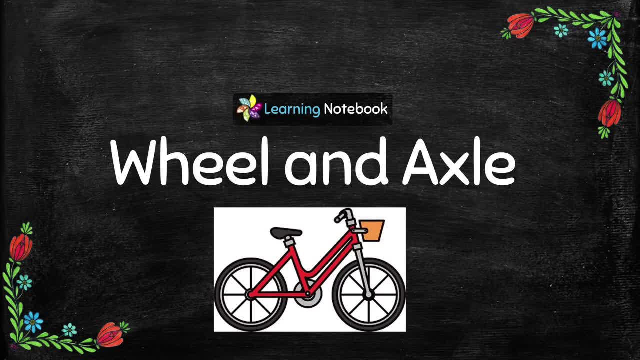 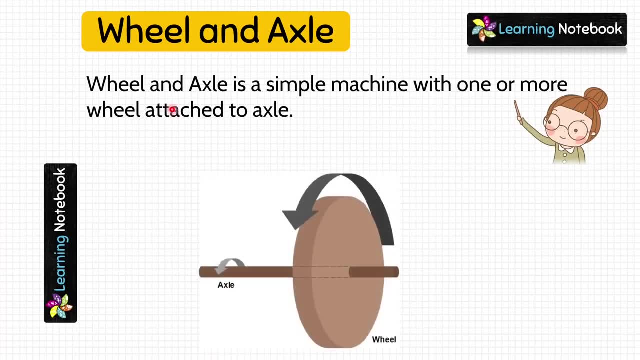 Now let's understand next type of simple machine: wheel and axle. Wheel and axle is a simple machine with one or more wheels attached to axle. Look here in this diagram, This is a wheel and this rod which is attached to the wheel is called axle. 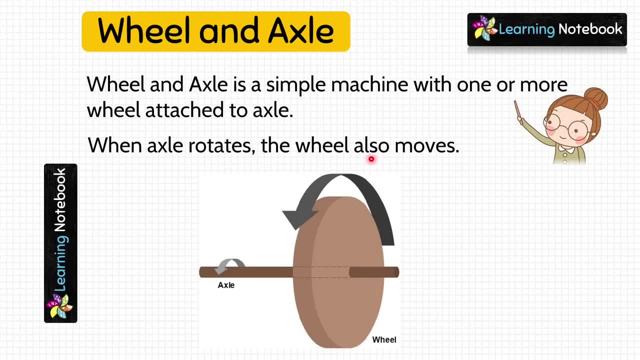 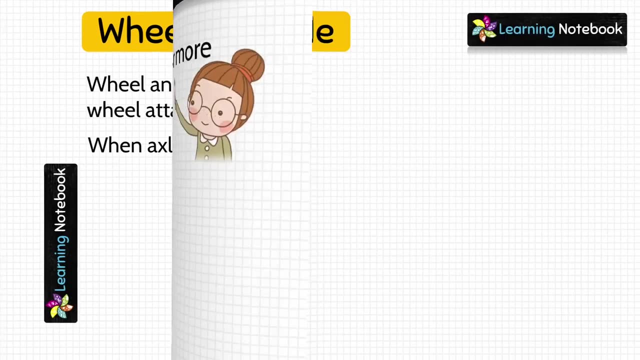 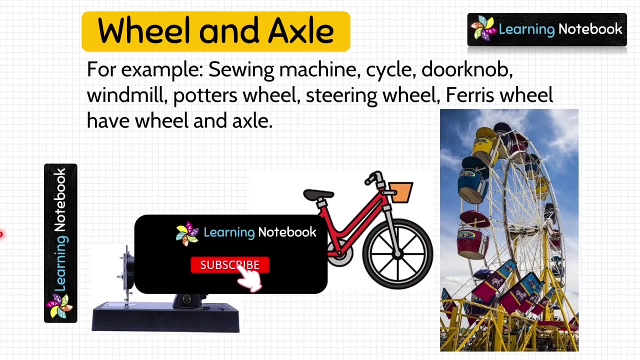 When the axle rotates, the wheel also moves, As shown in this diagram, And it requires much less effort to rotate an axle than to rotate a wheel. Let me tell you some examples of wheel and axle Swing machine: cycle door knob, windmill. 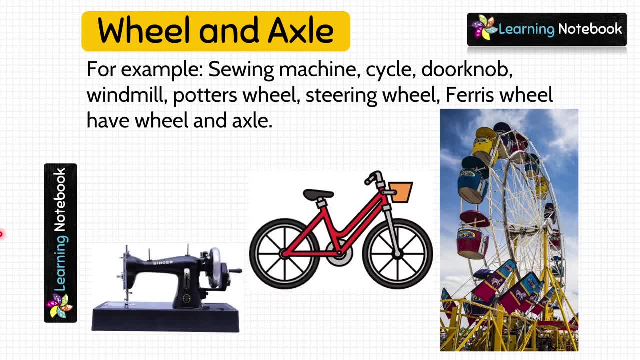 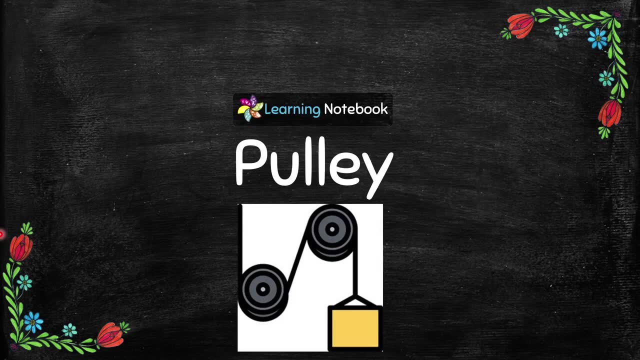 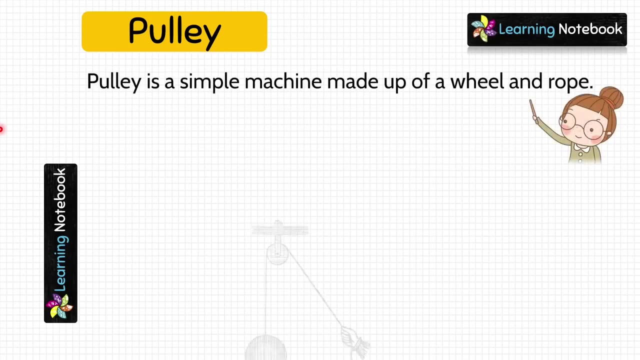 potter's wheel, steering wheel, ferris wheel- All of them have wheel and axle. So all of them uses simple machine, wheel and axle. Now let's understand last type of simple machine: pulley. Pulley is a simple machine. 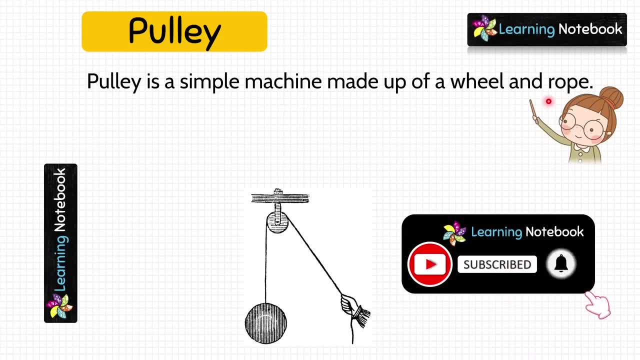 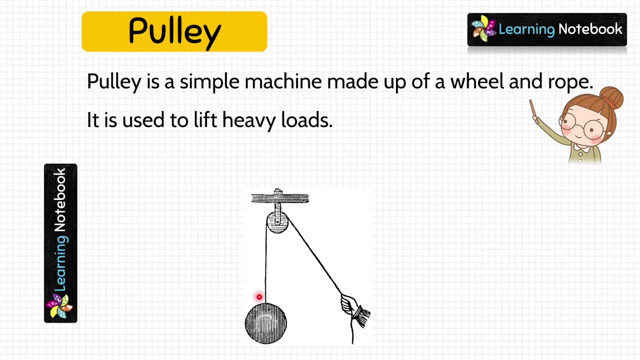 made up of a wheel and rope. It is used to lift heavy loads Students. if we lift a heavy load manually, it requires large amount of effort, But if we use pulley it takes very less effort to lift the same load. 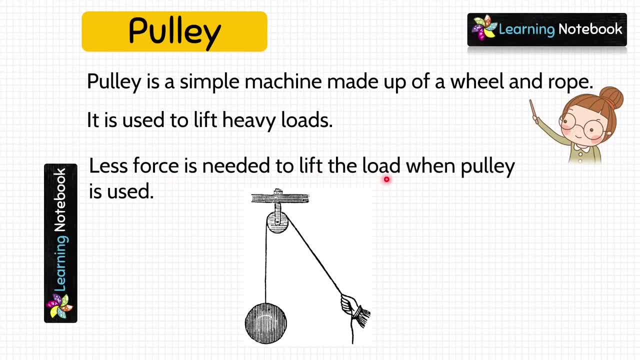 So less force is needed to lift the load when pulley is used. Now students look at this picture of pulley. There is a wheel on the top and there is a rope. Now one end of the rope is attached to the. 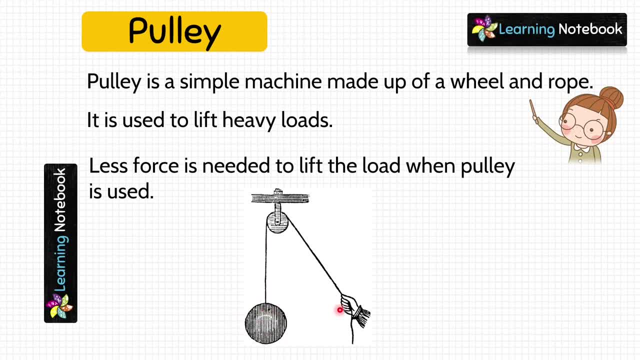 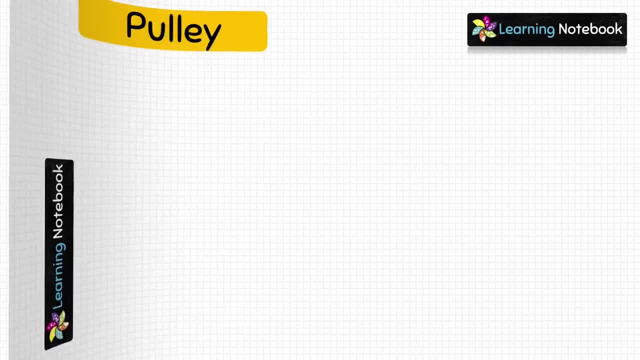 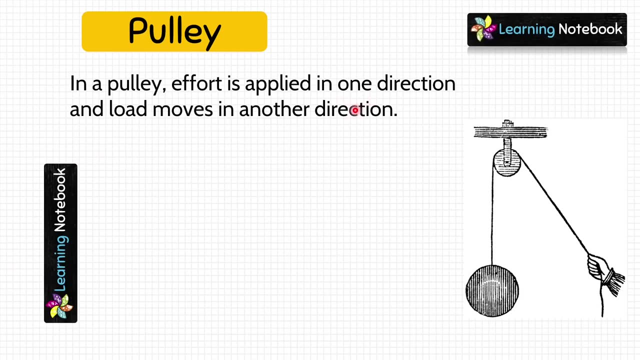 load And from other end of rope we put effort. So this is a pulley In a pulley, effort is applied in one direction and load moves in another direction, Like here: if we pull this rope in downward direction, then 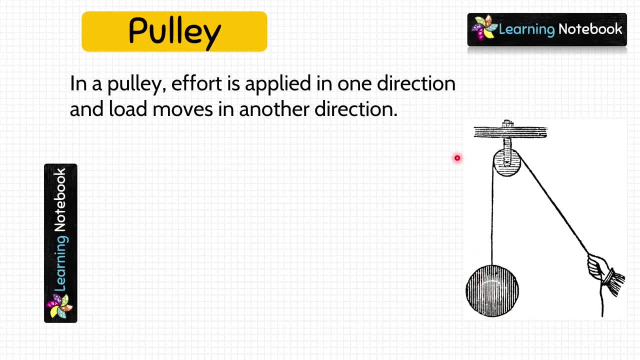 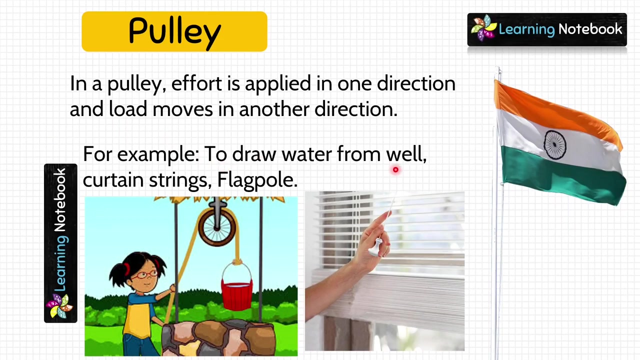 this load will go in upward direction. So in a pulley, effort is applied in one direction and the load moves in another direction. Now let's see some examples of pulley. We use pulley to draw water from well in the villages. 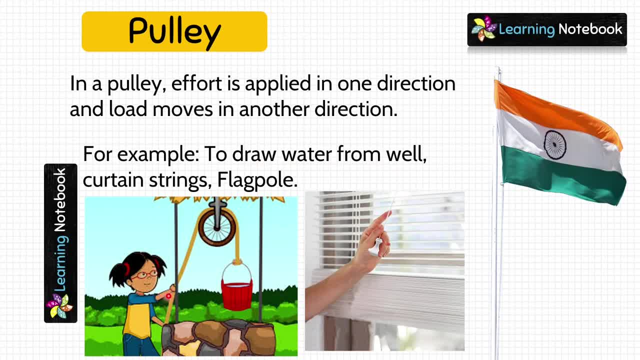 Look here, This bucket is the load, and when this girl pulls this rope down, then this bucket will go up and will draw water from well. So this is a pulley. Now, this is a pulley. You must have seen students curtain strings. 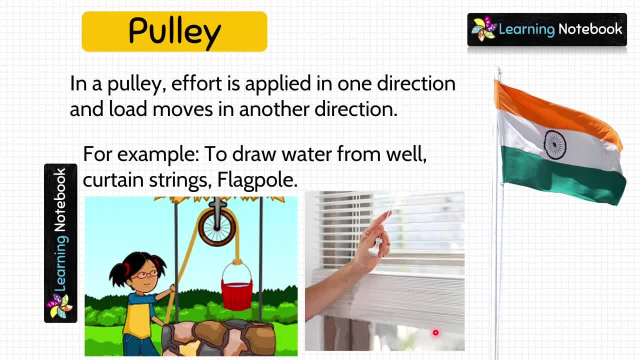 When we pull them down, these curtain strings move the curtain up, So they are also a good example of pulley. This flag pole is another example of pulley, because when we pull it moves the flag up. So all these are examples of pulley. 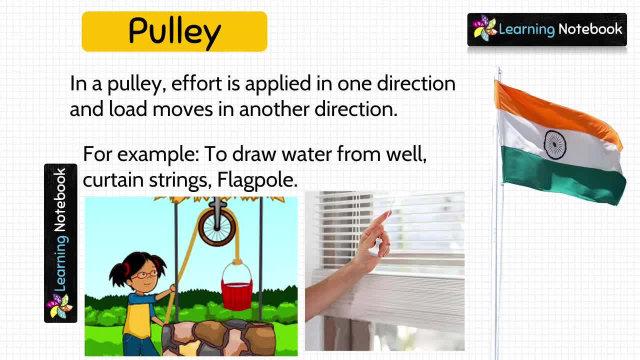 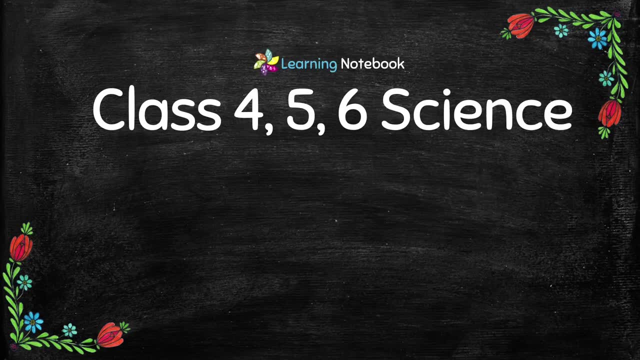 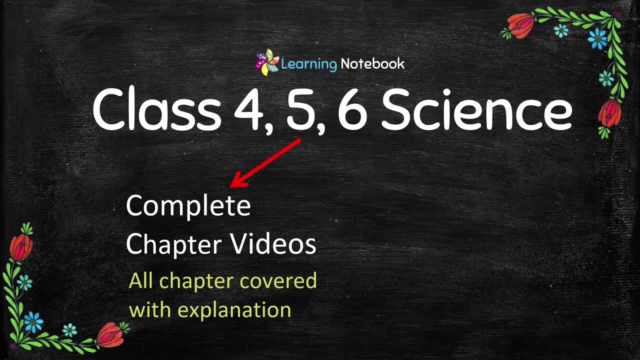 So now, students, I am sure you have understood what is simple machine and the types of simple machine, along with their day to day examples. Students, we would like to tell you that we have made videos on every chapter of class 4,, class 5 and class 6 science. 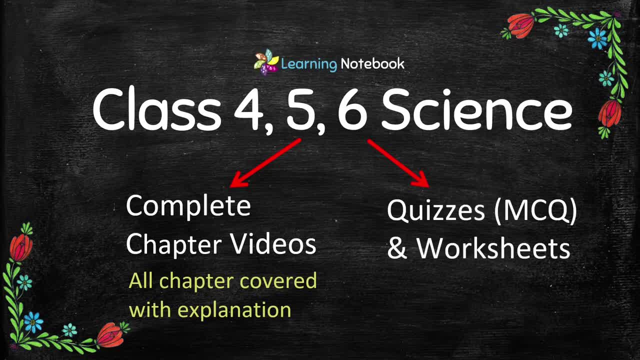 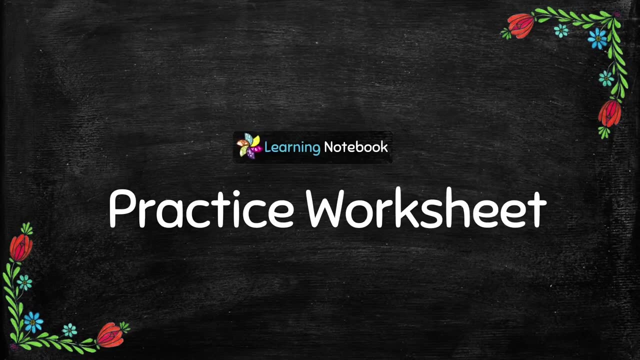 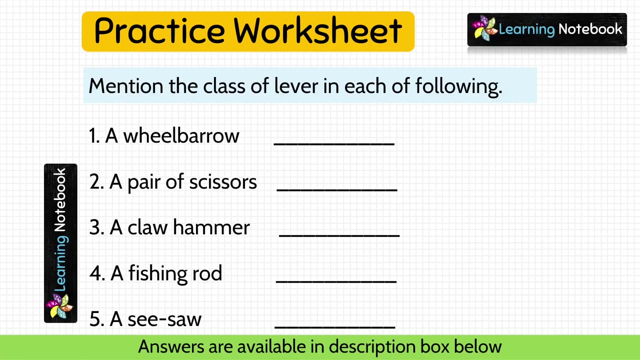 We also have interesting worksheets and quizzes on each chapter, So I would suggest you to check out our channel Learning Notebook. In the end, students, I am giving you a worksheet for your practice. This worksheet contains questions from all the sections of the chapter which I have just taught you. 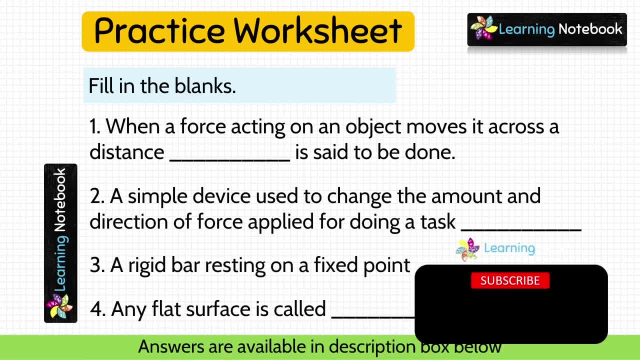 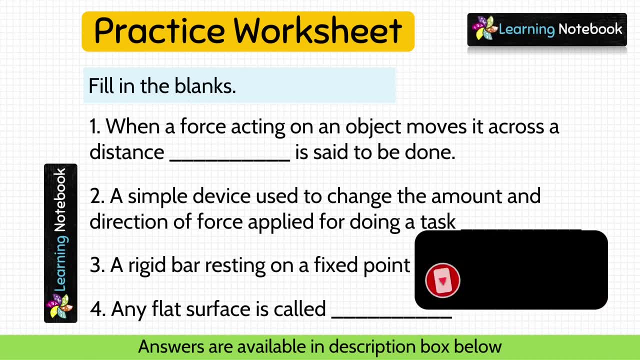 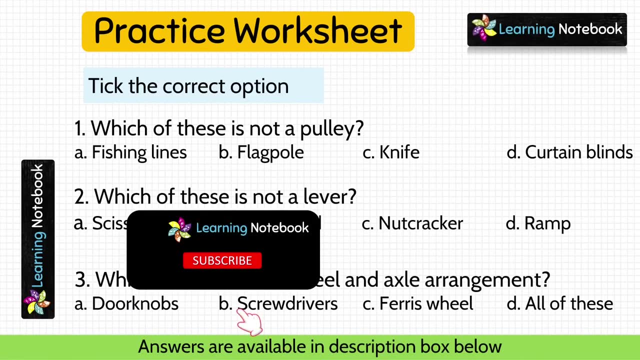 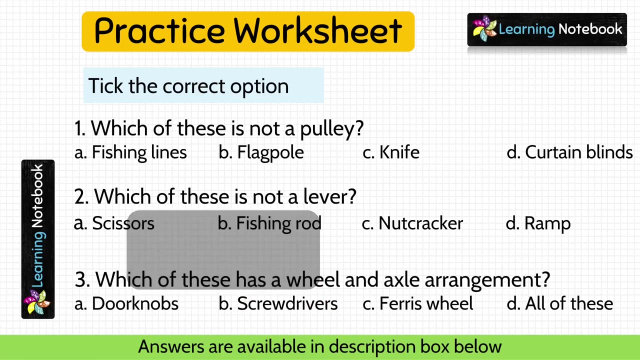 So, before attempting this worksheet, I would suggest you to first watch the video carefully. Do watch my other videos and share my channel and my videos with your friends and family. Thanks for watching. See you in the next video. Bye-bye, Thank you. 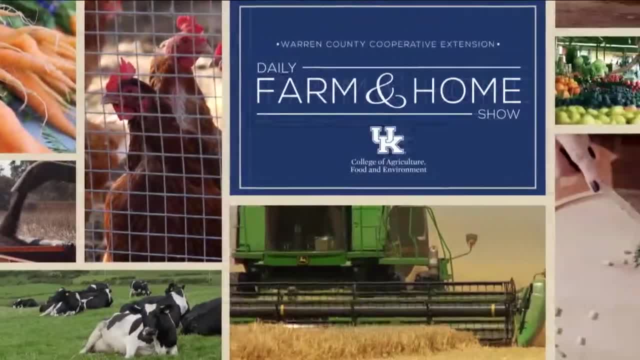 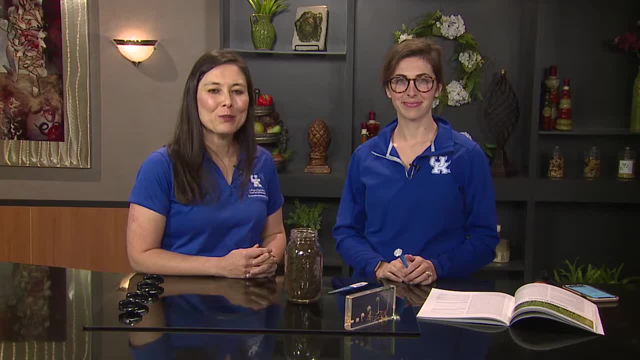 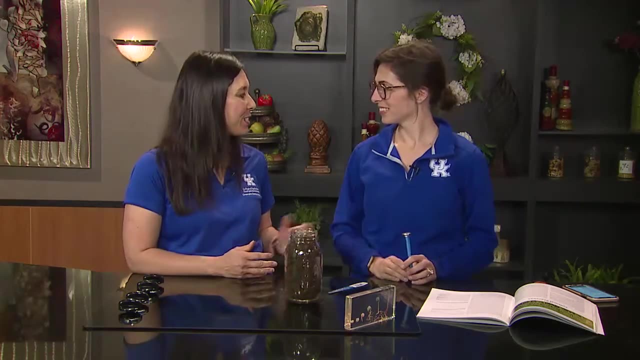 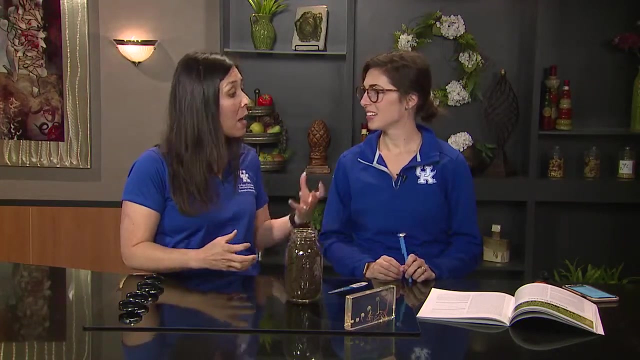 Good morning and welcome to your daily farm and home show, brought to you by the University of Kentucky Cooperative Extension Service. And now here's your host. Good morning and welcome to your farm and home show. My name is Joanna Coles, and this morning we're visiting with Camille Lambert. She's the Henderson County Extension Agent for Agriculture and Natural Resources. Good morning, Camille. Good morning, Well, I'm glad you're here today. Spring is definitely here. We already have some corn planted in Warren County. It's wild, isn't it? It is. The university has some recommendations about. 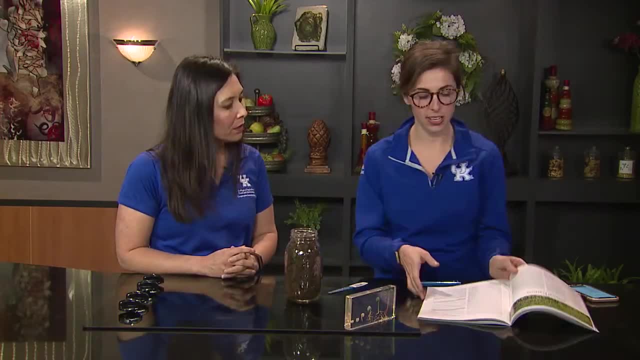 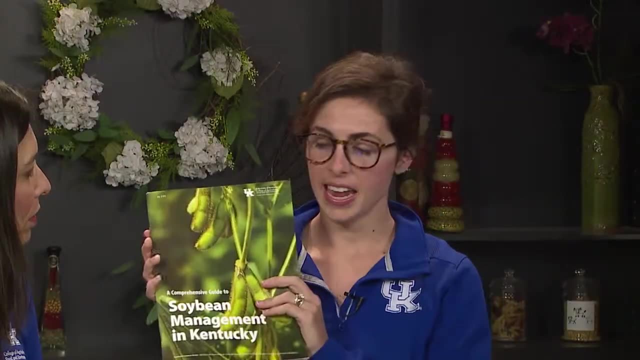 absolutely proper planting time, Sure, So they actually. the University of Kentucky just came out with this soybean management in Kentucky guide. It's brand new this year and it has tons of research-based information that you can use to make really good decisions when it comes to. 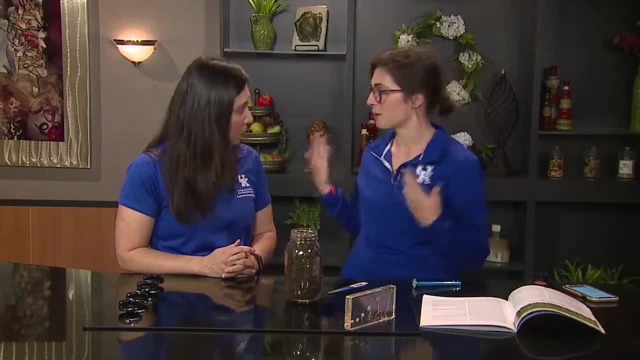 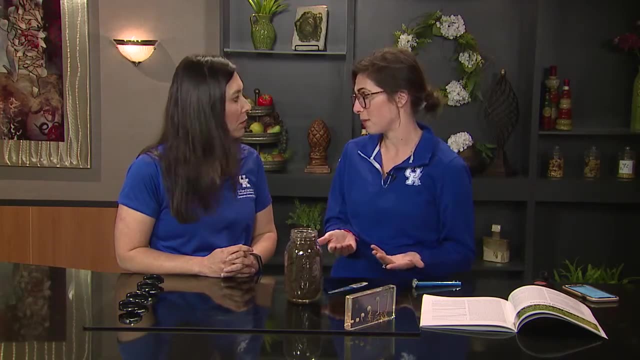 planting. So the first thing that I always like to discuss when I talk about planting with people is the soil temperature, because that is one of the most important things, aside from it being too wet, which we a lot of times will have this time of year. So do you know what this thing is? A thermometer? 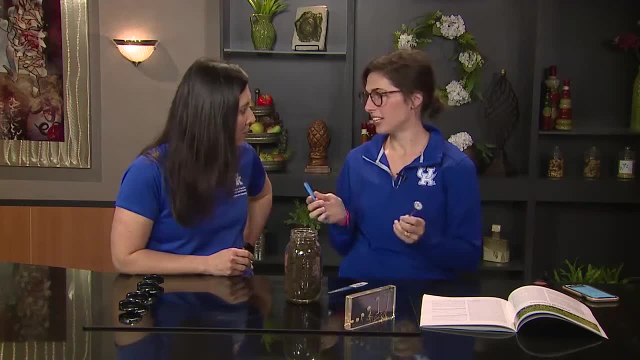 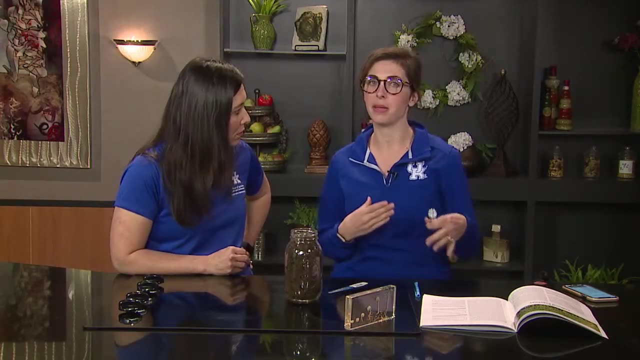 So I carry this thing around in my pocket daily this time of year, because it's essential that you check the temperature whenever you are making the decision. is it time for me to plant? yet? And the temperature can vary, you know, from Warren County to Henderson County, where I'm at, So you